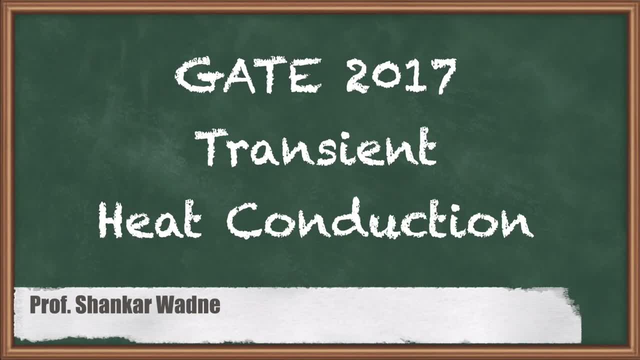 Hello, my dear students, in this lecture we are going to see one previous year GATE numerical. This question was asked in GATE 2017 for two marks in set 2.. Basically, this question is based on transient heat conduction, which is also called lumped heat capacity analysis. 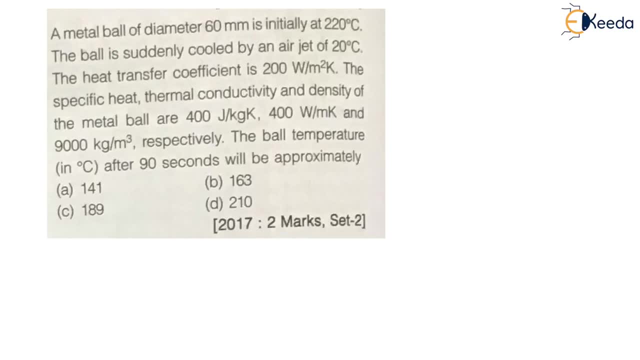 So let us understand the question. The question is a metal ball of diameter 60 mm. Now, my dear students, they have given a metal ball. Ball is nothing but spherical. So let us draw here a sphere, Let us say: this is a metal ball. 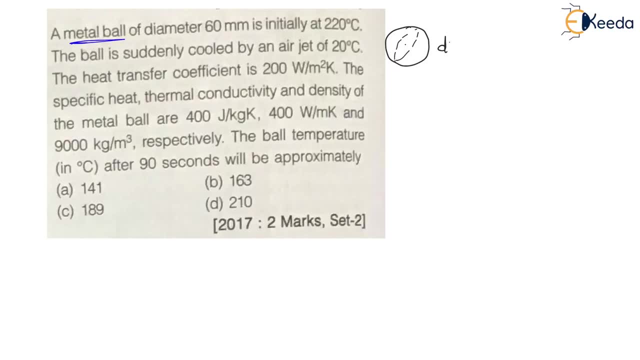 It is a spherical having diameter D. This is given 60 mm, Diameter is given 60 mm. Therefore, diameter is nothing, but we can say 60 into 10 to the power minus 3 meter Then is initially at 220 degree Celsius. 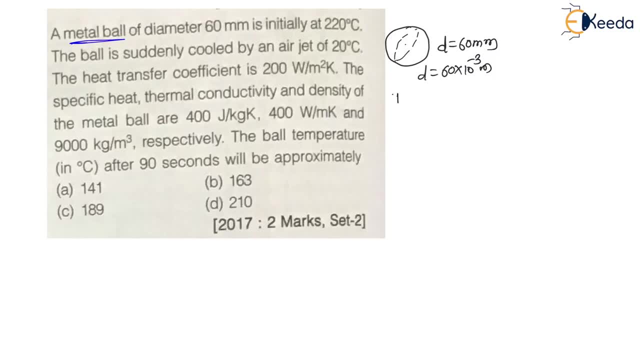 Now initial temperature of this metal ball is given. Therefore Ti is equal to 60. To 20 degree Celsius. Then the ball is suddenly cooled by air jet of 20 degree Celsius. Now air jet is nothing but surrounding fluid. Therefore the T infinity surrounding fluid temperature is nothing but 20 degree Celsius. 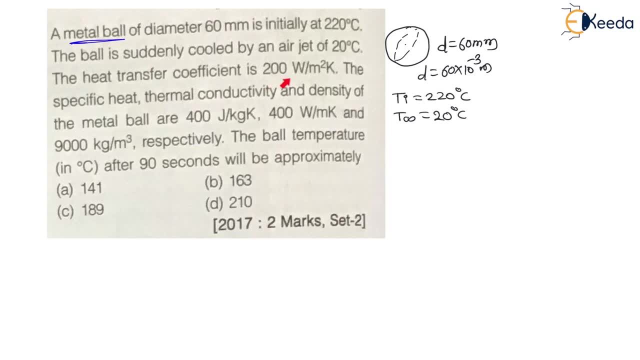 Then the heat transfer coefficient is 200 Watt per meter square Kelvin. Here convective heat transfer coefficient is given 200 Watt per meter square Kelvin. Then the specific heat, That is, Cp, thermal conductivity K and density, Rho of the metal ball are: 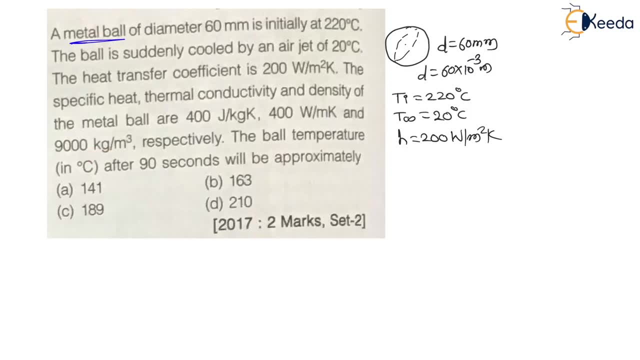 Now this is the specific heat Cp, thermal conductivity K and density Rho. So let us write down here Specific heat: Cp is given 400 Joule per kg Kelvin. Thermal conductivity K is given 400 Watt per meter Kelvin And density Rho is given 9000 kg per meter cube. 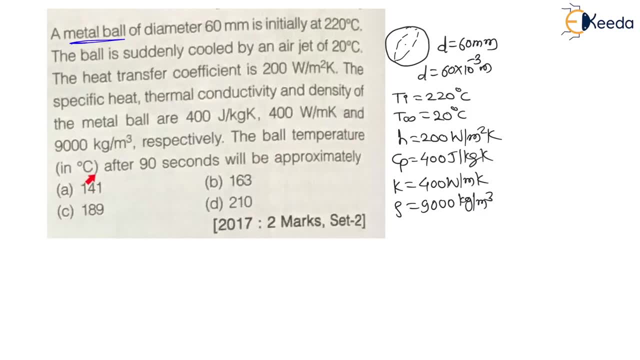 Respectively, The ball temperature in degree Celsius after 90 seconds will be approximately. Then, after 90 seconds- That is time is 90 seconds- We have to find the ball temperature in degree Celsius. Now, my dear students Here for such problems. 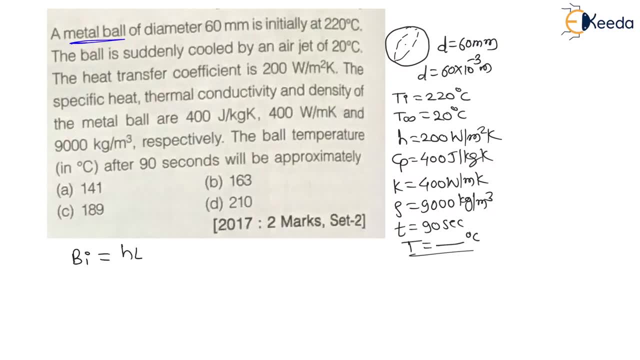 First of all we have to find biot number, And biot number is nothing but HL divided by K of solid, Where L is characteristic dimension. This L is calculated as H into volume divided by surface area of this object Divided by K. 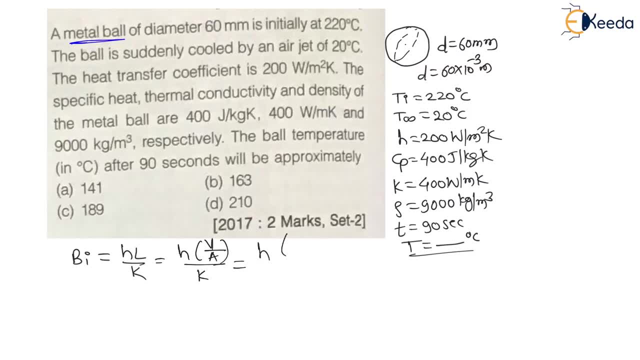 Right. Therefore, H is nothing but H. Volume of sphere is 4 by 3 pi R cube Divided by surface area of sphere is 4 pi R square Divided by K. Now, my dear students, Let us put here values to find biot number. 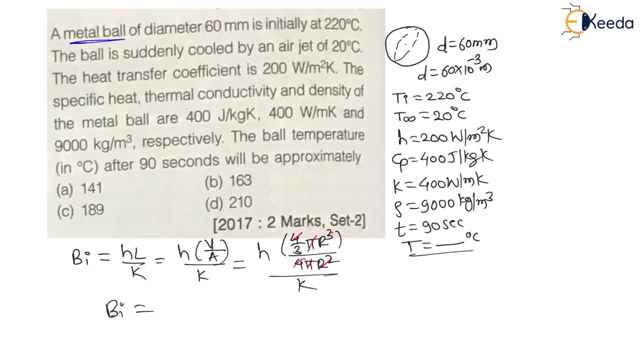 So here this 4, 4 pi, pi will get cancelled. R square- R square will get cancelled And the final resulting formula will become That is, H into R divided by 3 K. So let us put the values. Therefore, H is given 200 into. 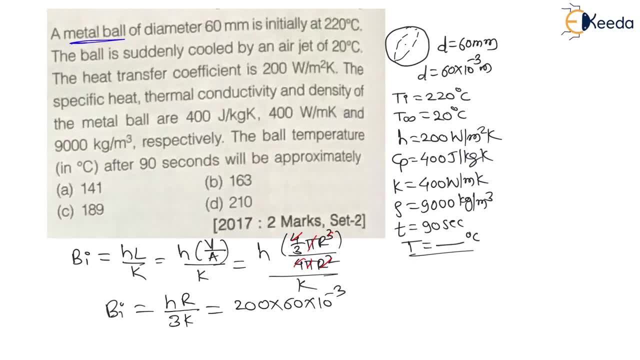 R is diameter divided by 2.. Therefore 60 into 10 to the power minus 3.. Divided by 2 into 3, into K, is nothing but 400.. If I solve this equation, I will get 5 into 10 to the power minus 3.. 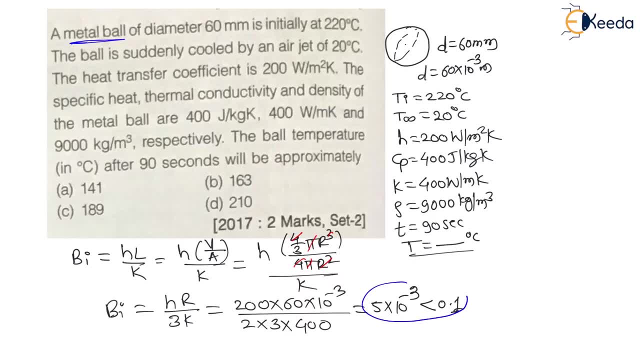 This value is less than 0.1.. So, whenever value is less than 0.1. The lumped heat capacity analysis is valid. So, my dear students, For this problem We are going to use lumped heat capacity analysis. Now, here, as per this lumped heat capacity analysis, 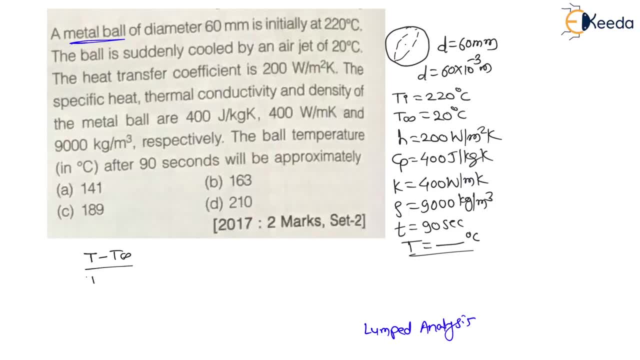 Temperature T minus T infinity Divided by T. i minus T infinity Is equal to T to power minus H A Divided by rho V C, T into time, T Right. This is the formula for finding any unknown With the help of lumped heat capacity analysis. 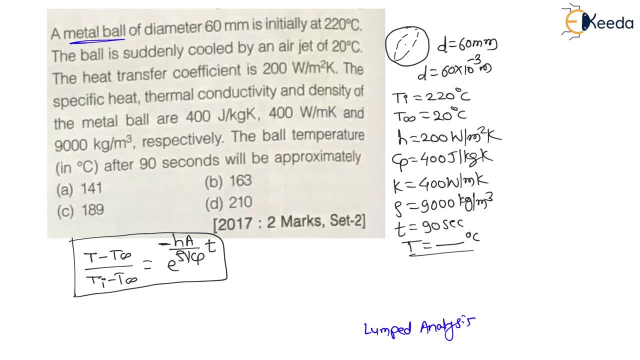 Where T is the temperature after some time. T- T- infinity- is the fluid temperature. T i is the initial temperature of this metal ball. H is convective heat transfer coefficient. A is the surface area of this metal ball. V is the volume of this ball. 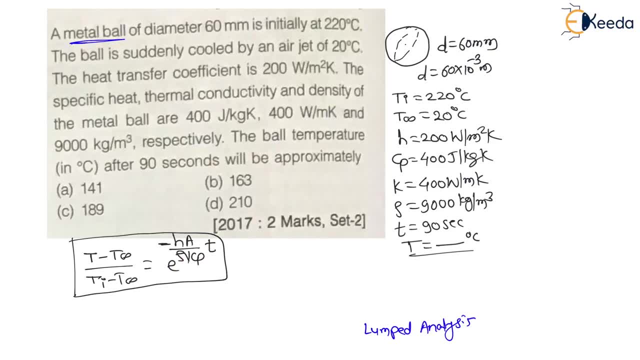 Rho is the density, Cp is the specific area, constant pressure, And T is the time. So, my dear students, Here T is unknown, So let us put the values. Therefore, if I put values T minus T, infinity is given 20.. 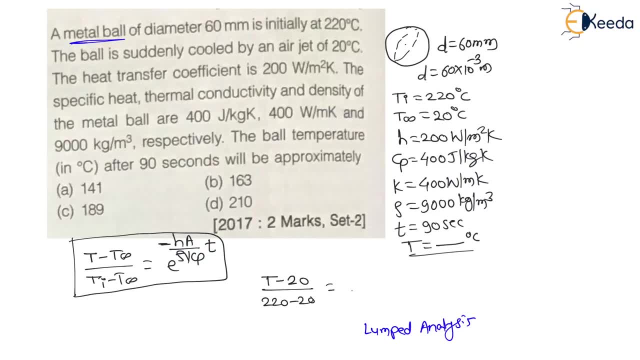 Divided by T, i is 220 minus 20.. Is equal to E, to the power, Minus H. A Divided by rho, V, C, P into T. Now here, This area, you have a volume of a sphere As it is given, sphere. 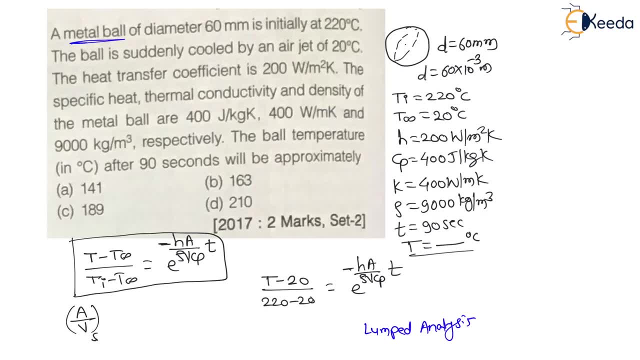 Therefore, this area you have, a volume Of a sphere, is nothing but Area of sphere is 4 pi R square. You have a volume is 4 by 3. Pi R cube. So here This 4 pi, 4 pi will get cancelled. 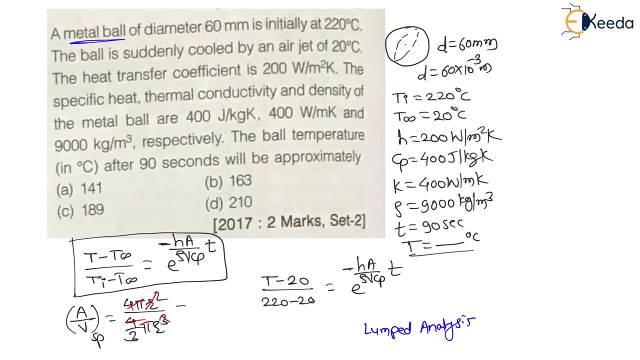 R square. R square will get cancelled. It will become 3 by R. It will become 3 by R, Right, Where R is small r. we have written here Right. Therefore, L by R, 3 by R. Now, my dear students, 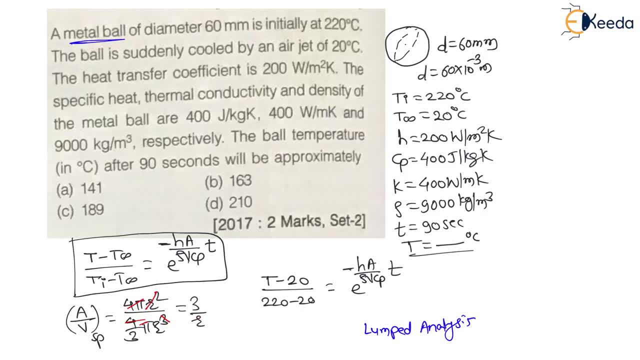 R is nothing but diameter divided by 2.. Therefore, it will become 6 divided by diameter d Right. So here, Instead of this Area divided by volume, Let us replace this area divided by volume With diameter 6 divided by diameter. 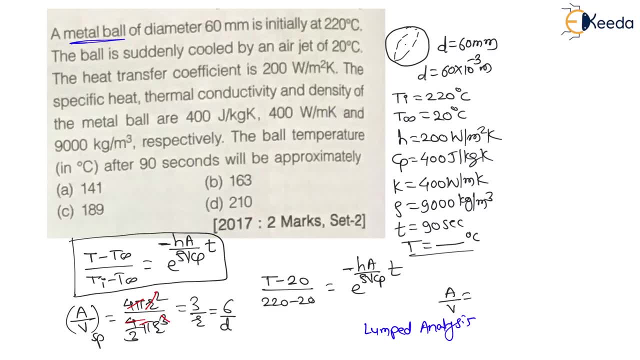 Therefore, Here I am replacing area divided by volume With 6 divided by diameter Right. So rewrite the formula Here. the formula will become This: formula will become T minus T infinity. T minus T infinity Divided by: 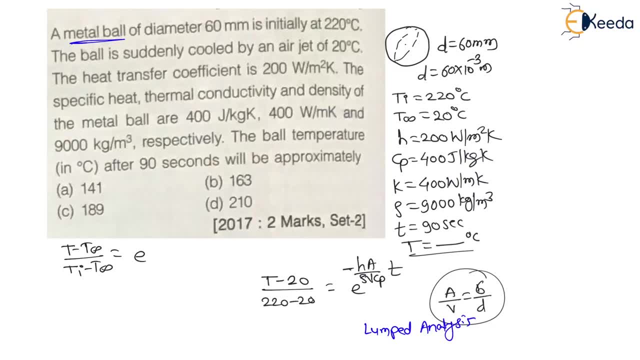 T, i minus T, infinity Is equal to T, to the power Minus H. t Divided by Rho, C, p Into Area divided by volume is 6 by D Right. So, my dear students, 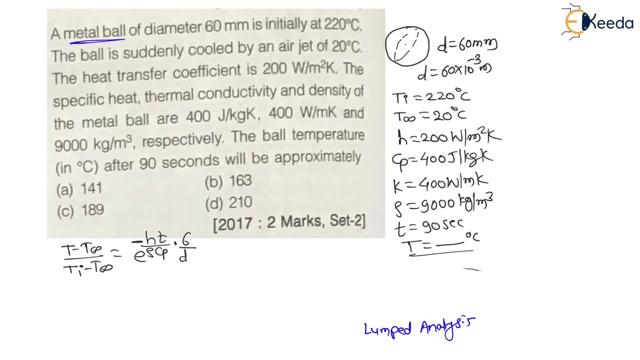 Let us put the values over here. If I put values, Then I will get the respective value. Therefore, T minus T infinity. T minus T infinity is 20.. Divided by T, i is 220.. Minus 20.. 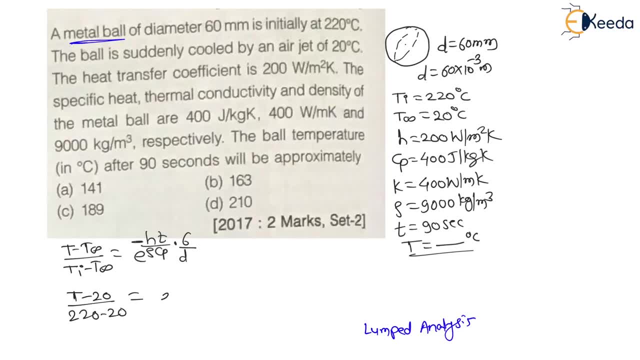 Is equal to T to the power Minus H t. Therefore, T to the power Minus H, H is nothing but 200.. Into time is given 90, second Into 6.. Divided by Density is given: 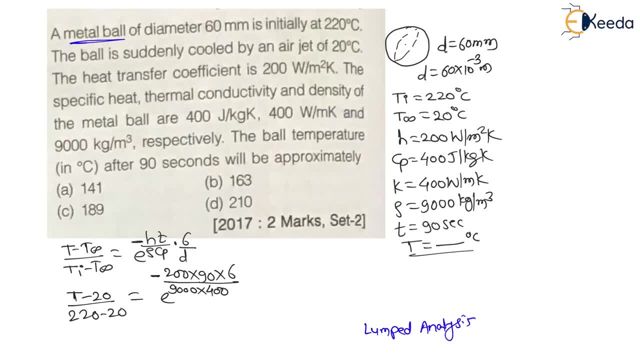 9000.. T p is given 400.. Into diameter is given 60 into T, to the power Minus T. Right Now, in this complete equation, My dear students, Only T is unknown. So let us simplify this equation.